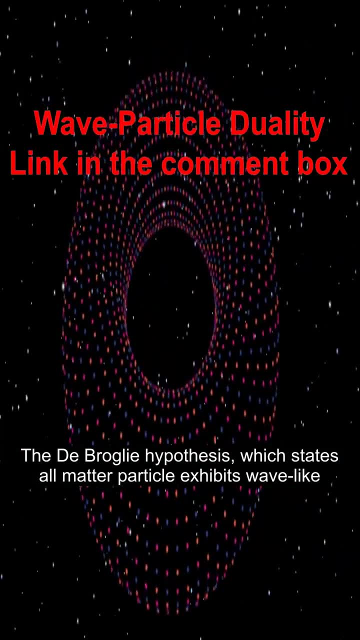 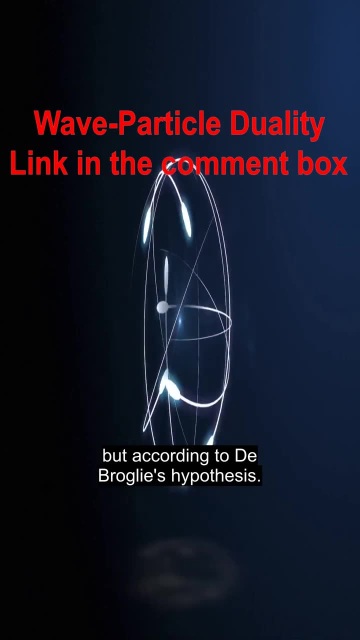 The de Broglie hypothesis, which states all matter. particle exhibits wave-like behavior and waves exhibits particle-like behavior. Electron has definite mass, position and velocity, but according to de Broglie's hypothesis, electrons can behave like waves, which is one of the main. 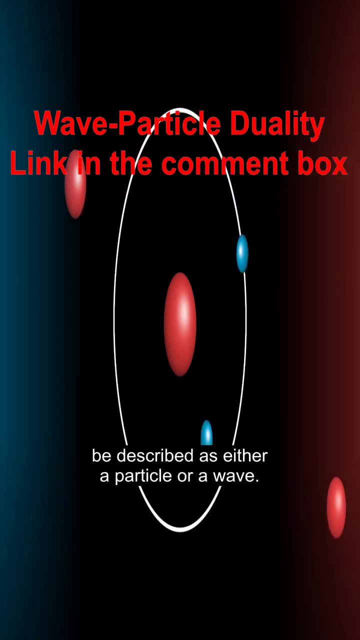 concepts in quantum mechanics that every particle may be described as either a particle or a wave. 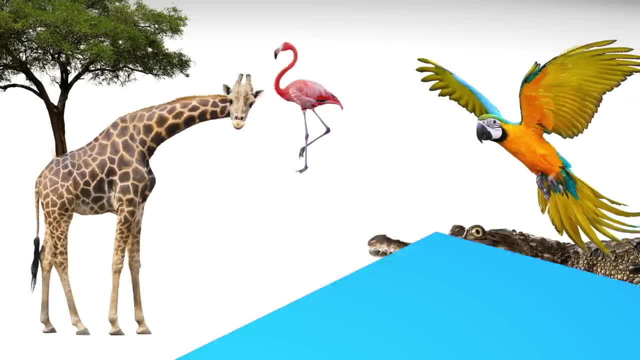 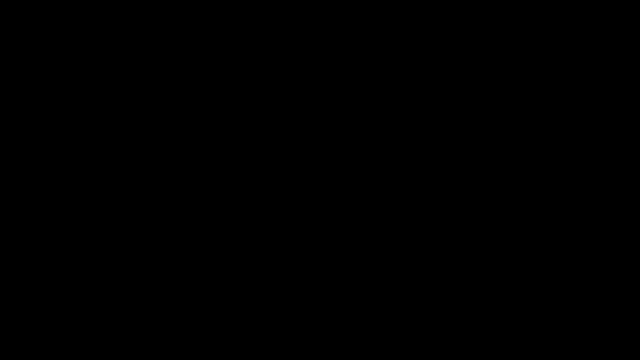 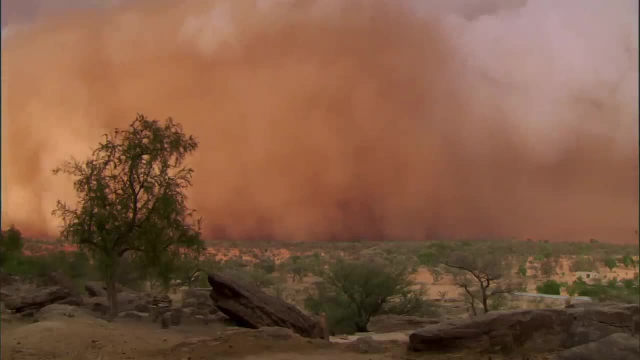 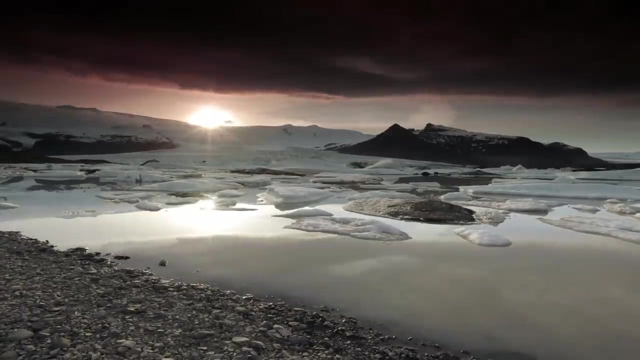 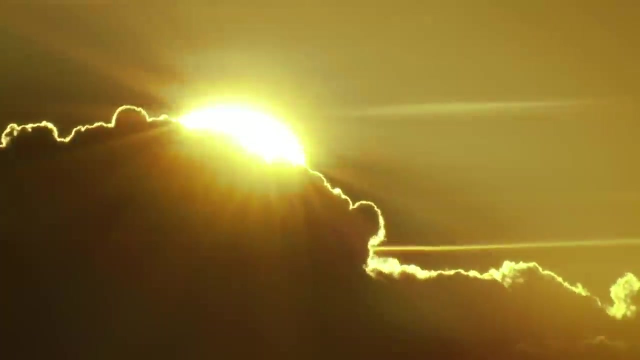 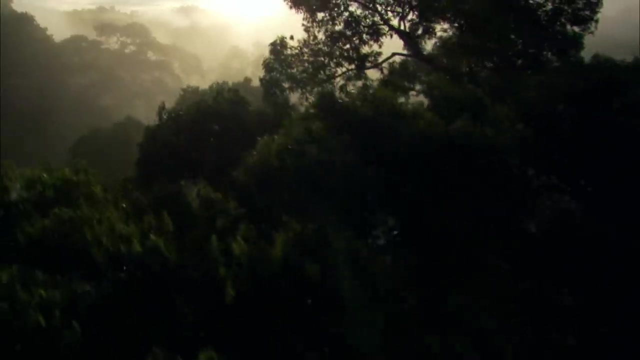 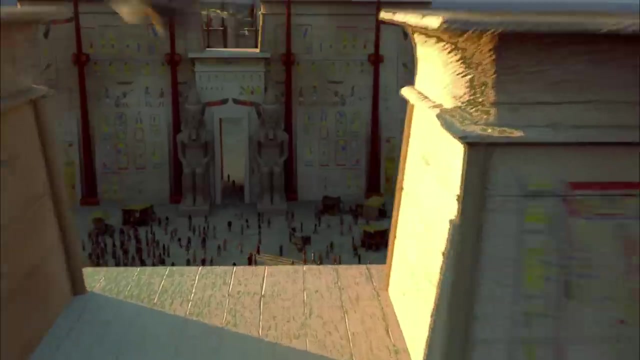 Freezing cold, oppressive heat, devastating drought. Extreme climate change may have contributed to the extinction of the Neanderthals and allowed modern Homo sapiens to dominate the Earth. All life on Earth is subject to the power of climate. Civilisations evolve or vanish forever. 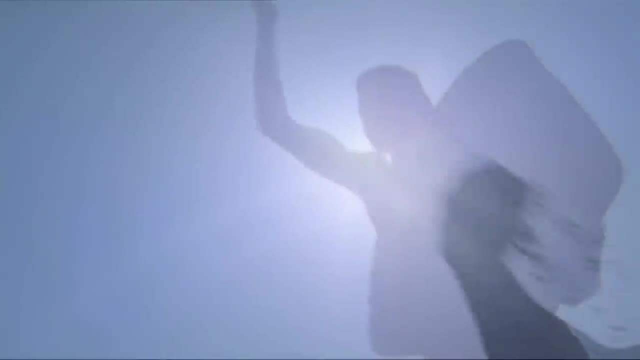 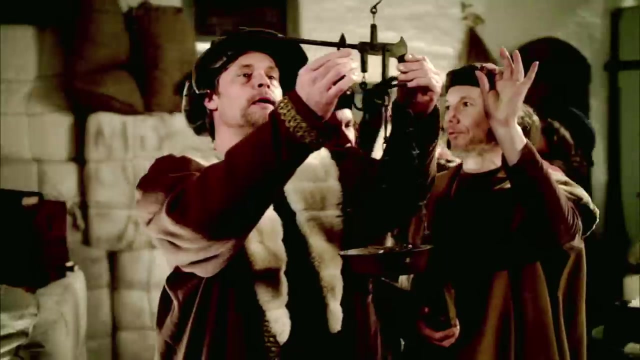 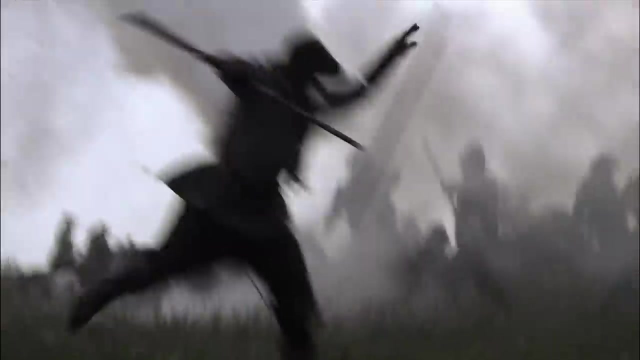 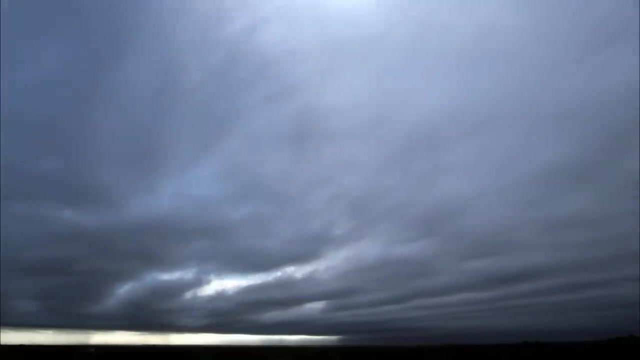 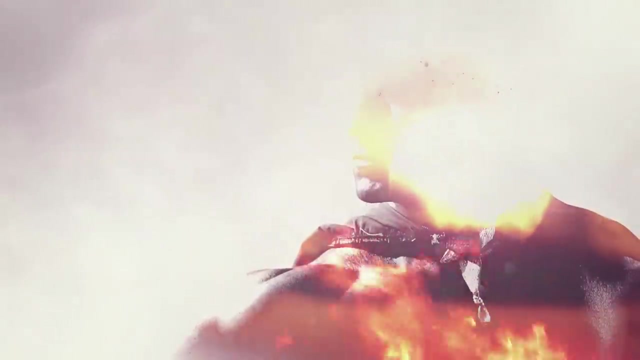 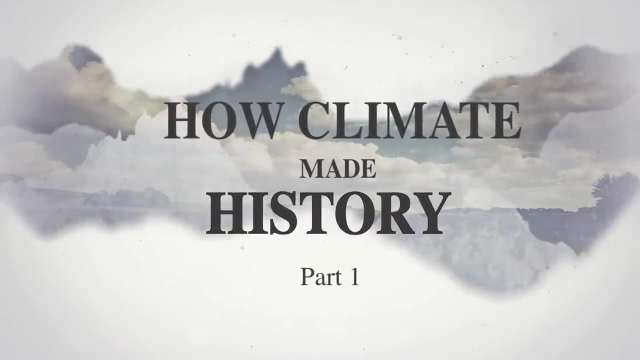 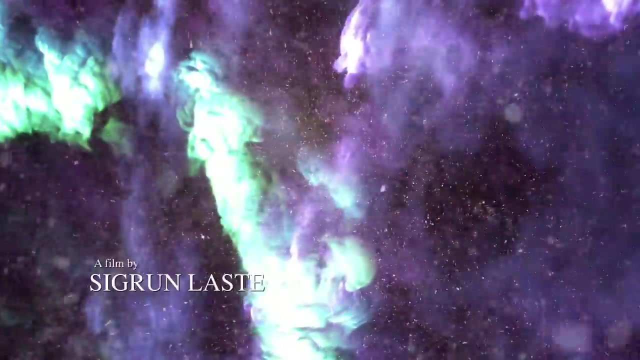 Favourable climatic conditions support the rise of great empires and promote trade, prosperity and artistic achievement. Adverse climatic events often lead to war and other human catastrophes. But what about the future? Almost 14 billion years ago, immense forces created the universe. 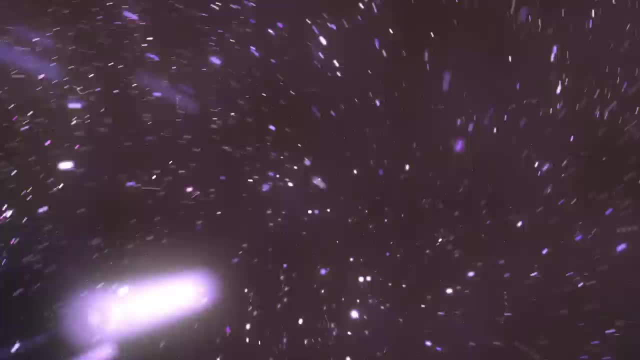 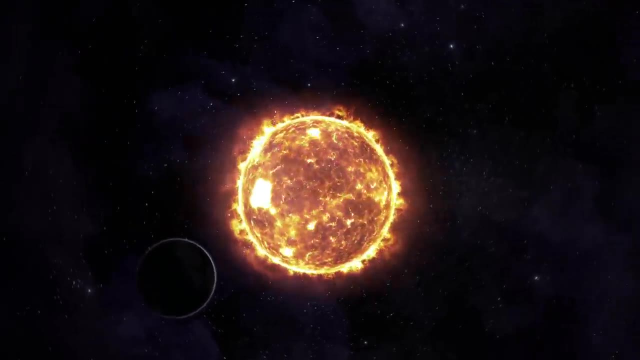 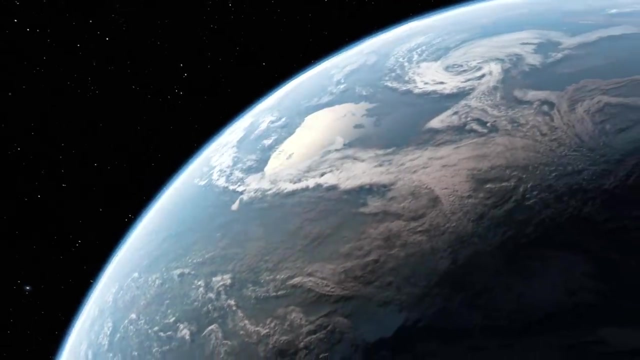 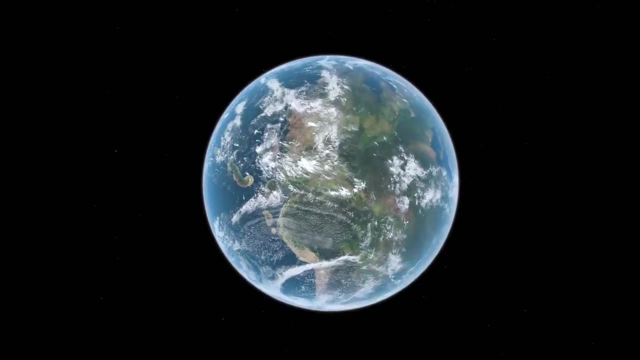 The Big Bang spawned vast galaxies, each with millions and millions of stars, moons and planets. Among these is one small blue planet: our Earth. Water, warmth and the Earth's protective atmosphere create something that may be unique in the universe: A climate that makes life possible.